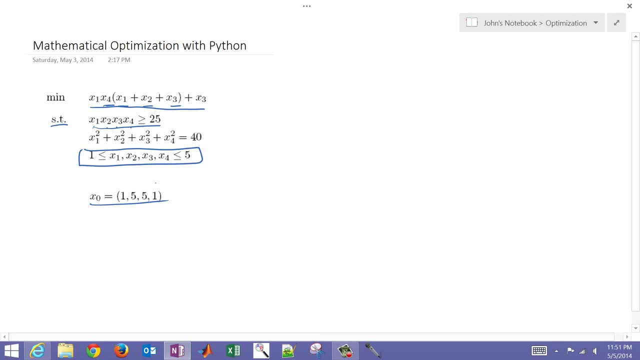 this is going to be the starting point for the numerical optimization for each of those x1 through x4.. x1 is going to equal 1, x2 5, and so on. So we're going to use Python to be able to. 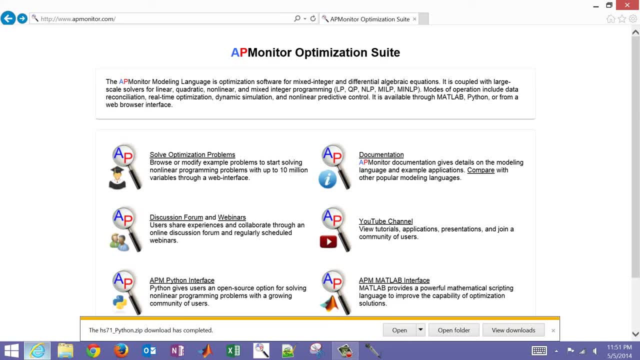 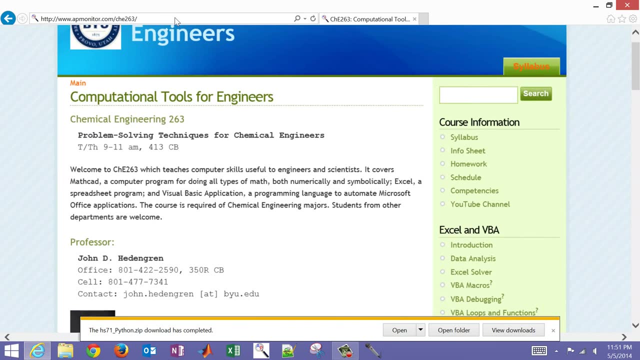 solve this problem. And first of all, if you just come to the apmonitorcom website and then when you get here, you can either follow the link for the course or type in CHE 263. And this will bring you to computational tools for engineers. And we previously solved the same. 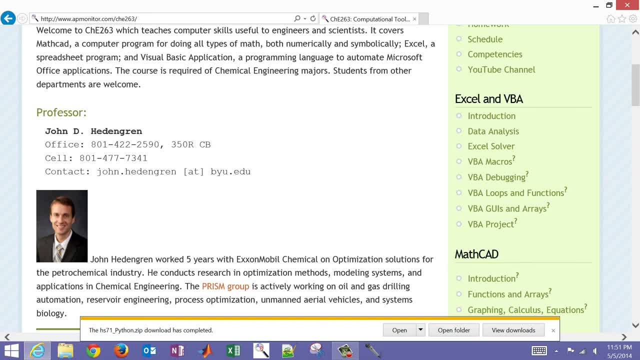 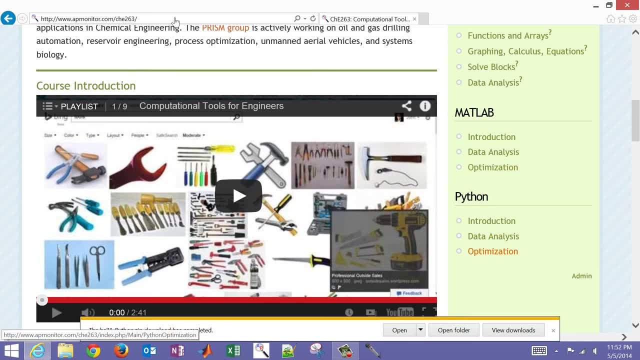 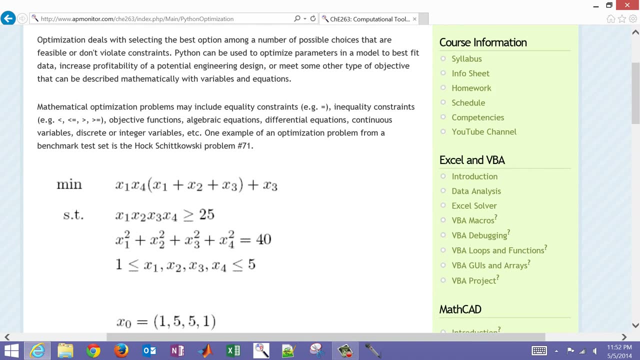 problem with the Excel solver And you can see on the right hand side in the Excel section and then also in the MATLAB section, the same problem. We're going to visit the Python one this time. Okay, so if you come down on the Python script you'll see: download this benchmark problem. 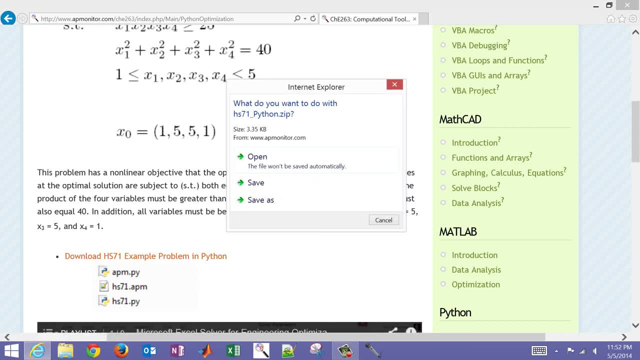 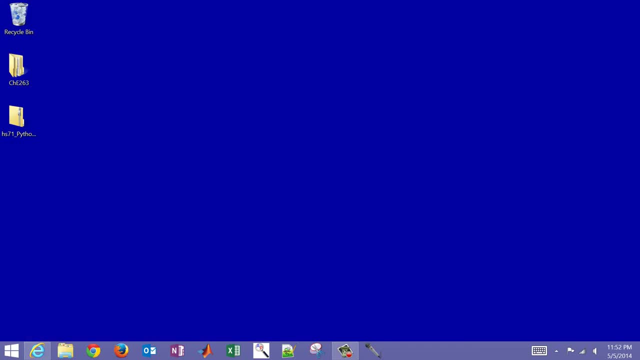 just 71. And if you select that link, it'll allow you to save it. I'm just going to save it to my desktop in this case, and come back over and extract that. So the first thing we need to do is: 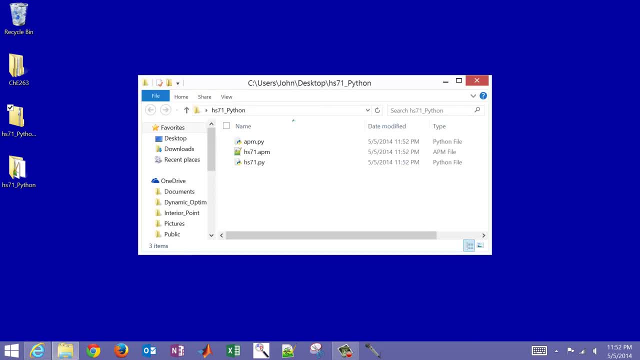 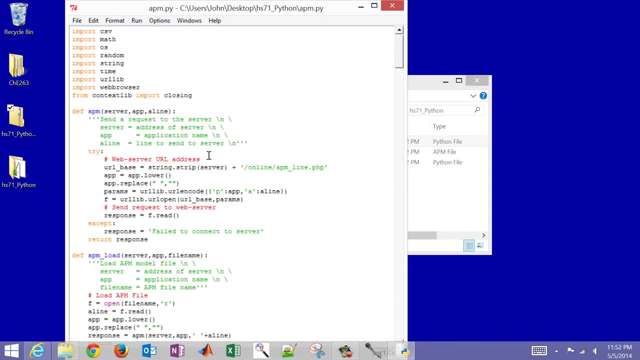 just extract these files And you'll see when it opens up. you'll see four files. The first file: if we just go ahead and open that with the IDLE editor, you'll see that this is something we don't need to change. These are just the AP monitor. 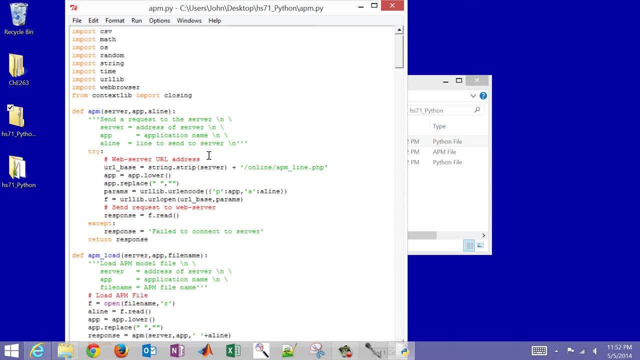 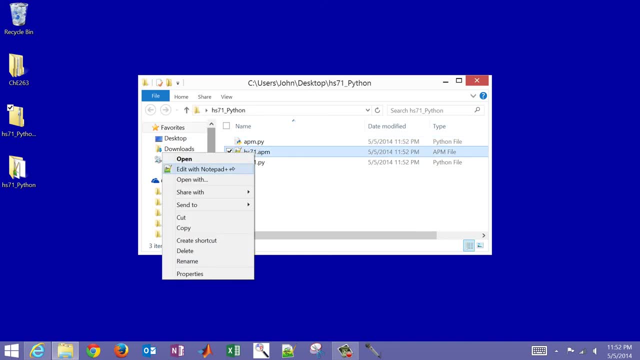 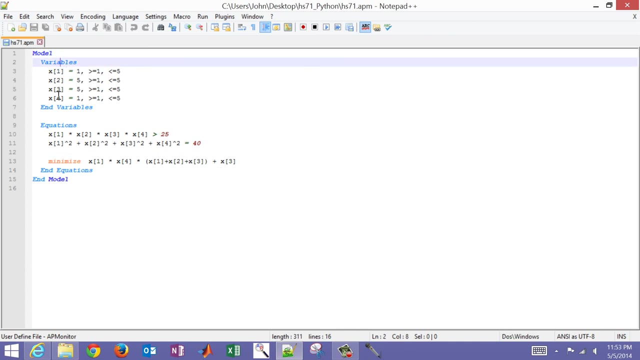 interface files, the source code to be able to access the optimization routines. The next file that we have, this one you can open up with any text editor. I'm going to use Notepad++ for this, with the syntax highlighting. I have my four variables: X1 through X4. And you can see that the product of those 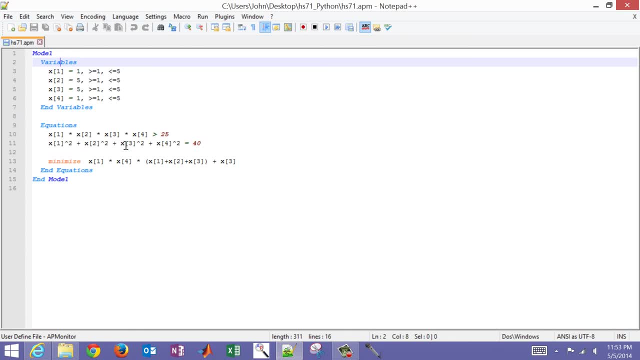 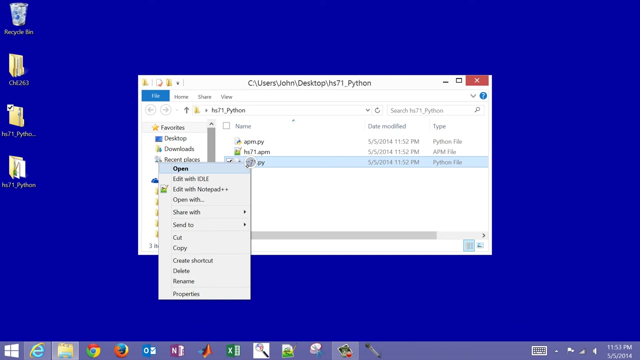 is greater than 25.. And then the sum of the squares of those has to equal 40.. Finally, I also have my minimize objective function there. Okay, so that is the model file, And then let me open up the script file. This is what we're.